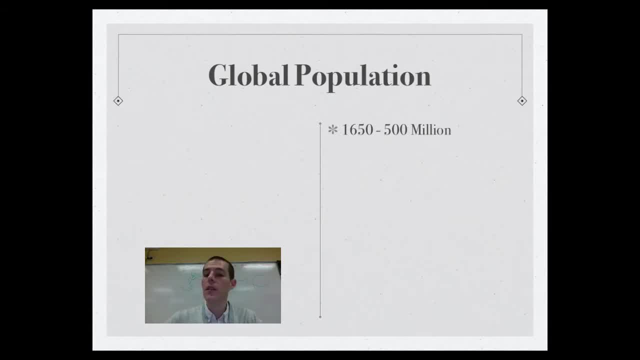 an increase in the quality of life for people. So 1650, you got 500 million people on the earth. Jump forward 200 years and we have doubled the population to 1 billion people. and then, after this point, things really start to pick up. So jump forward a short 80 years: you have doubled. 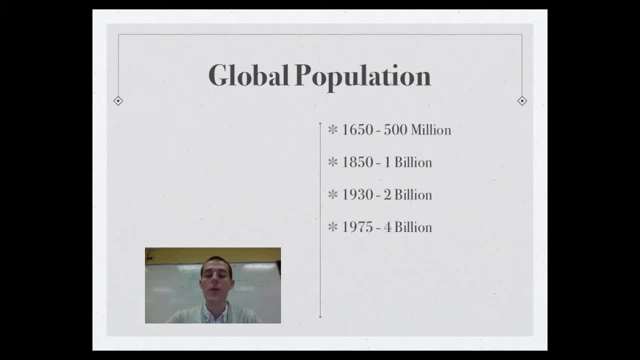 the population again to 2 billion people. Jump forward another 45 years and we are at 4 billion people. and here we stand in 2013 at 7 plus billion people. So human population grew exponentially. for quite a long time It peaked like peak. population growth rate was somewhere around 2.2%. 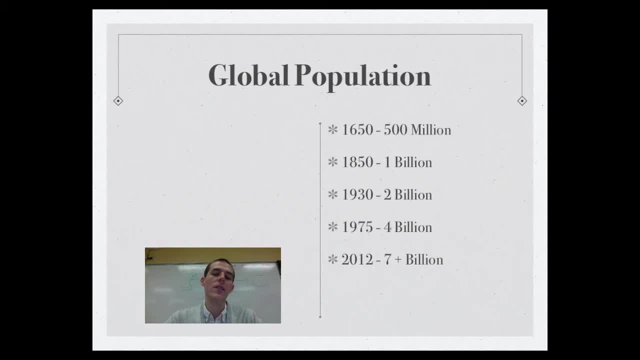 per year in the 1960s. It's since decreased to 1.5 to 1.7% per year, which is still a very rapid growth rate, but it looks like the human population has grown over time. So let's start out with a. 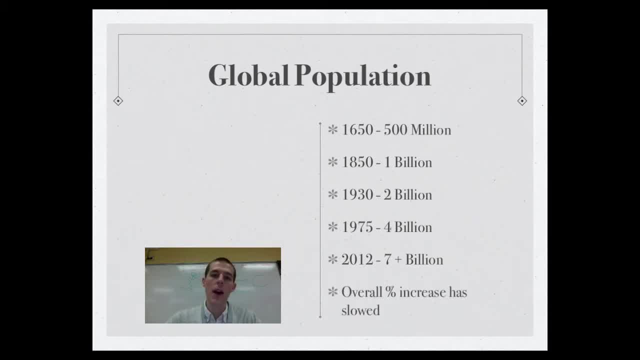 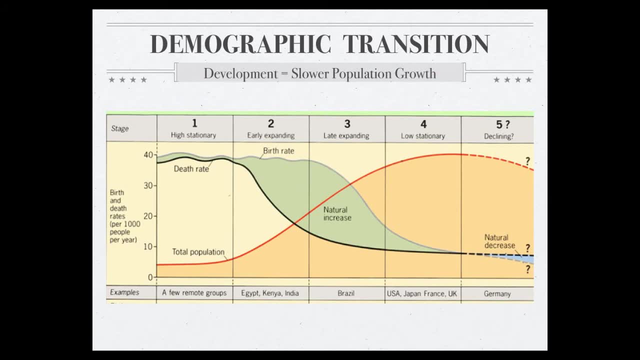 little bit about population growth. So the population has stepped off of the exponential part of the graph. Now, talking about human population growth, I want to introduce you to a model called the demographic transition, And the demographic transition basically talks about how population growth in a country changes as the development of that country increases, going from the most. 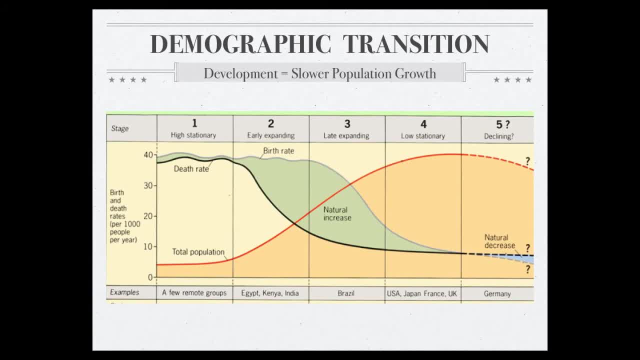 basic, rudimentary of society, all the way up to a highly industrialized, very advanced society. So let me walk you through this a little bit. There's some very interesting things that you can see. So, in a stage, one country, and this is- 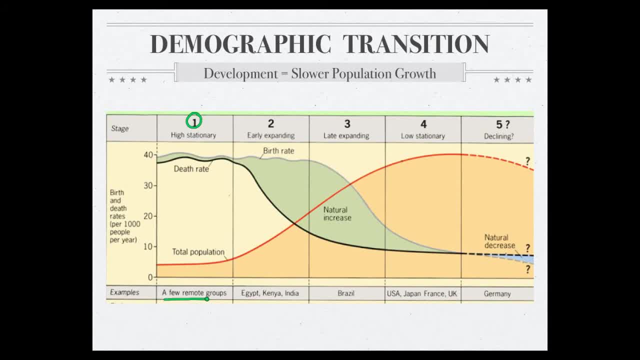 represented by a few remote groups, probably living as nomads or in the deepest jungles in a stage one society. you've got a very high death rate, black line and a very high birth rate And your total population isn't growing very quickly, because the idea essentially is that if you've got a lot of 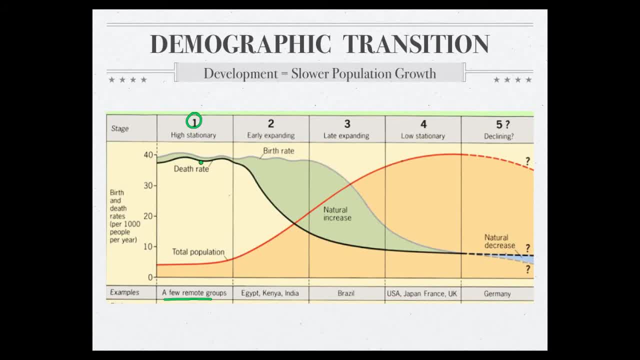 children dying off, you also need to have a lot of babies to replace them. So things stay pretty. I don't know. I guess pretty even As that country starts to develop and becomes more advanced. they're known as an early expanding society. Examples of this: Egypt, Kenya, India. 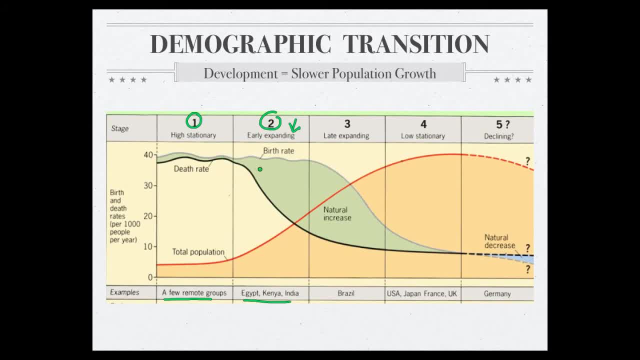 In this part of the demographic transition, we see the death rate starting to decrease quite dramatically because the quality of life is improving, Sanitation's improving, medicine's improving, So people are dying much less frequently. However, particularly people still think, hey, I need to have a lot of kids in order to make sure that they 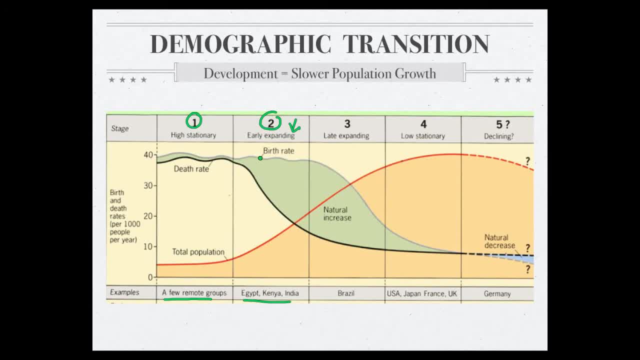 make it into adulthood. So, though death rate's decreasing, the birth rate is still pretty high, which means that your population is going to start to grow pretty rapidly. at this stage Now, at a late expanding country, the death rate has fallen quite a lot. We also see the birth rate. 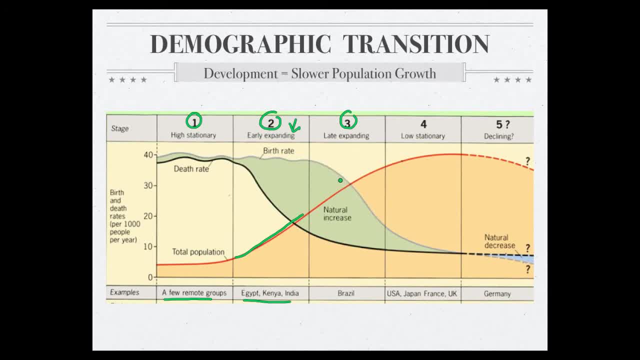 starting to fall off. So this is where culture starts to catch up with the reality of death rate. You start having development for women, You start seeing family planning options coming in. So that's what's taking our birth rate way down. And because birth rate still is fairly high and the death rate 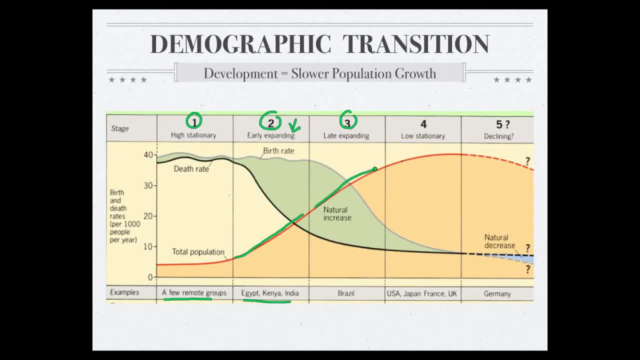 is pretty low. we're still increasing our population pretty rapidly. And then stage four country which is most of the developed countries in the world. you got US, Japan, France, UK. The population growth has pretty much leveled off because your birth rate has come down, your death rate is pretty steady and your 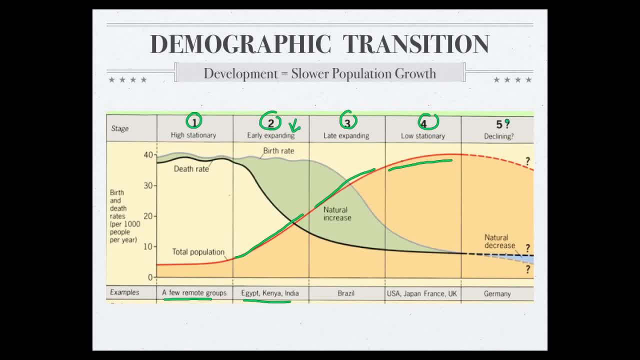 population is going to start to fall off. So that's what's taking our birth rate way down. And because birth rate actually has stabilized. And then right out here, stage five, demographers are still waiting to see whether there is truth in this model. But it's possible that these types of countries the birth rate has. 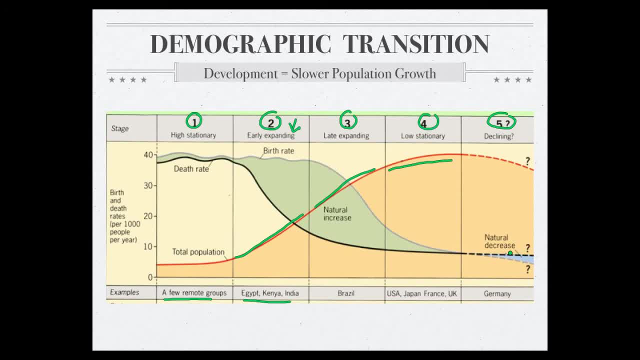 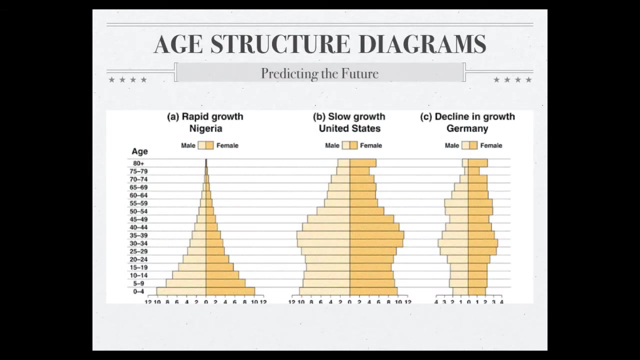 actually fallen below the death rate, So they are below replacement level fertility and the population is actually declining. An example of this would be Germany. Some Eastern European countries- Japan- are seeing this sort of transition presently, where they're seeing their population is actually starting to slowly decline. Another model: I want to show you that demographers 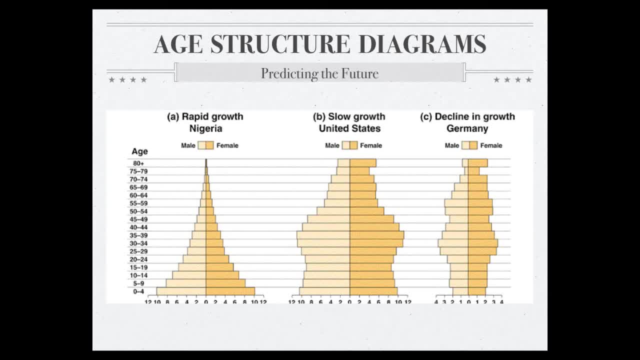 use to kind of look towards the future of a country. it's called an age structure diagram And an age structure diagram is basically a breakdown of the population in a country where you've got this graph split in half- males on one side, females on the other side- It is broken up by five year age blocks from birth all the way. 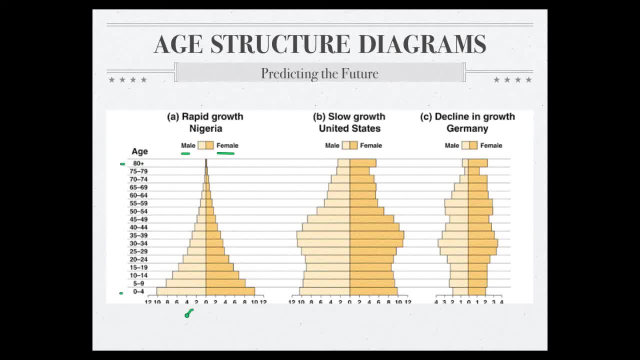 up until 80 plus years of age And the bottom is the percentage of the population that each bar represents. So you can see right here this pyramid shape is seen in a lot of developing countries And the thing that demographers can tell from this sort of 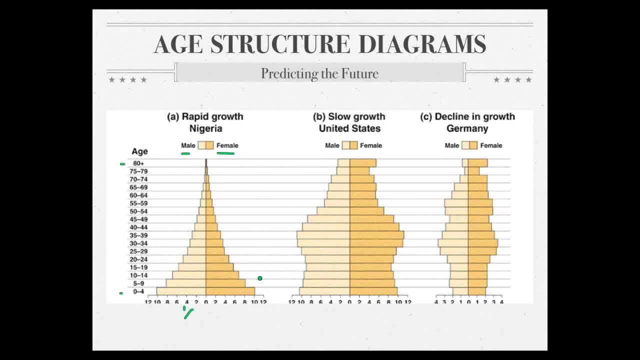 pyramid is that the population is going to probably grow very rapidly going forward because the bulk of your population- you can see the bigger part of your graph- is down here in their pre-reproductive and early reproductive years. So all of these people right here as these, through those flows, as they develop, they're going to see this kind of 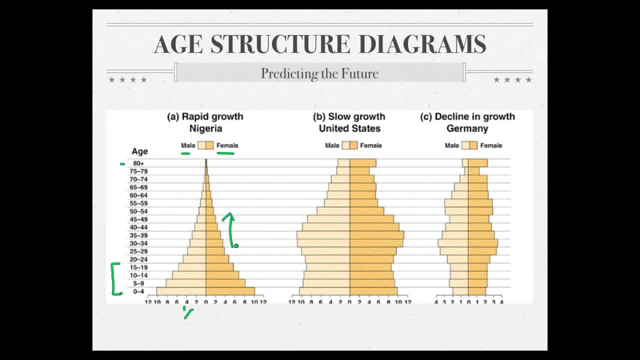 chunks of the graph move up, they are going to leave bigger pieces of the pyramid behind them, because all of these babies are having babies, so you're going to see rapid population growth in this sort of age structure. united states is an example of a fairly stable age structure diagram. 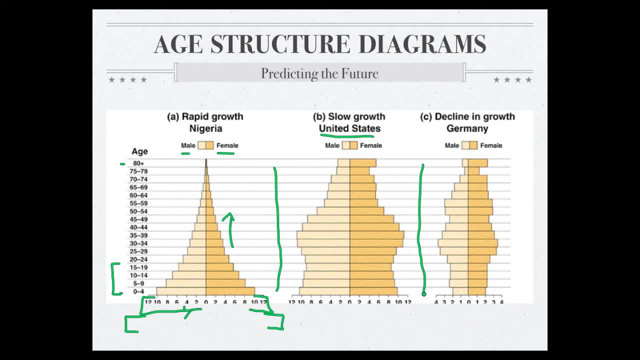 now. one thing to note with america that we currently face is we've got a large portion of our population right here in the middle. this is the baby boom generation, and as they move up into their older years, they're going to leave a smaller proportion of, i guess, americans below them, and 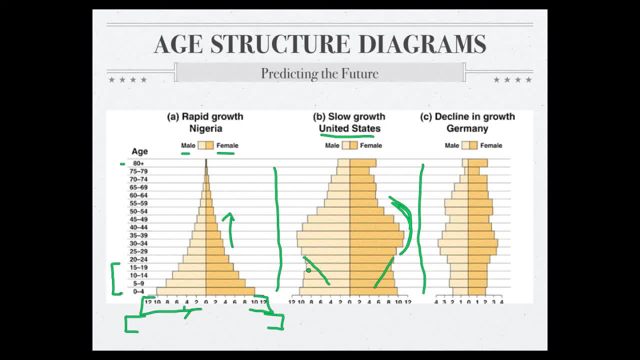 with social structures. set up the way they are, these working age people are paying into the social support systems that are taking care of this older generation. so a lot of people worry that, since the older generation is a bigger proportion of the population than the younger generation, they're going to have to pay more and more to take care of their older generation. so 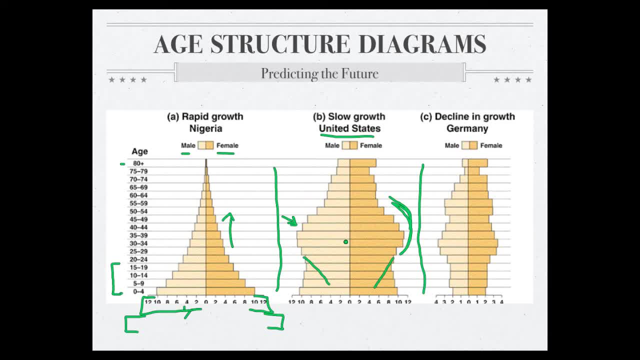 the programs that take care of this generation may not be financially viable. and then, in a declining growth model, you can see something that looks like this, or even kind of like an inverted pyramid, where you have got the largest proportion of your population up here, smallest proportion down here, which? 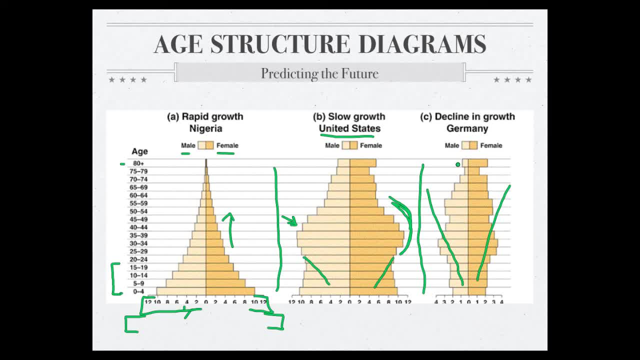 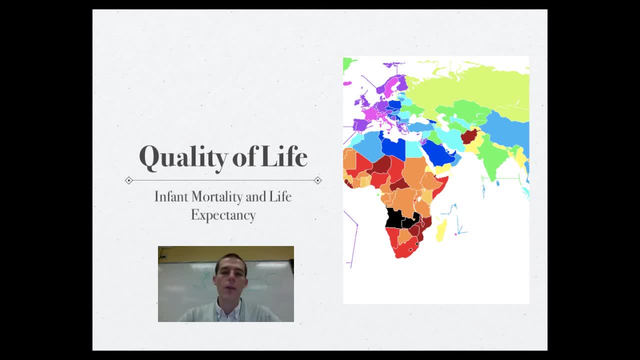 tells a demographer that the population of this country is going to be declining over time. a couple other qualities of population that demographers talk about is the quality of life, and that is basically looking at the infant mortality and life expectancy. so how many babies make it past the age of one? 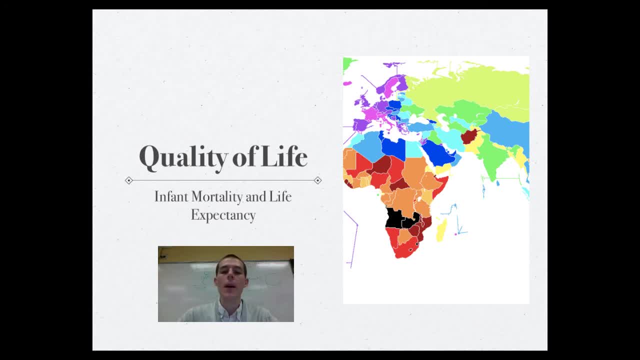 or two years and how long can't a person expect to live now? the map there on the right is showing colors based on expected life expectancy, and red is a very poor life expectancy. green to blue is pretty good life expectancy. so in countries that are developed they got a lot of medicine, a lot of opportunity. 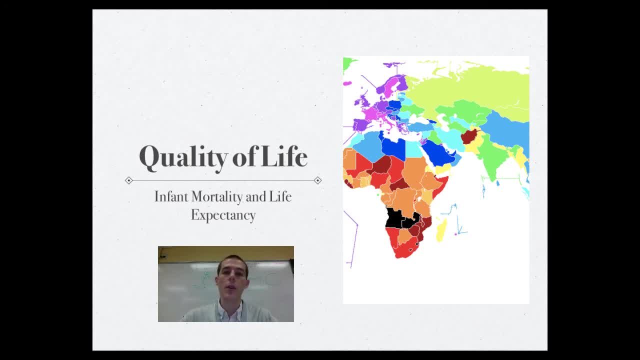 infant mortality is going to be pretty low and life expectancy is going to be pretty long. now, in a country that doesn't have some of those structures in place- a less developed country- infant mortality rate is going to be pretty high and life expectancy is going to be pretty short. so, based on the development of the 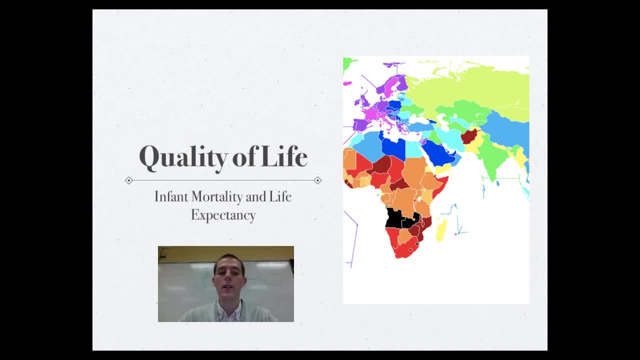 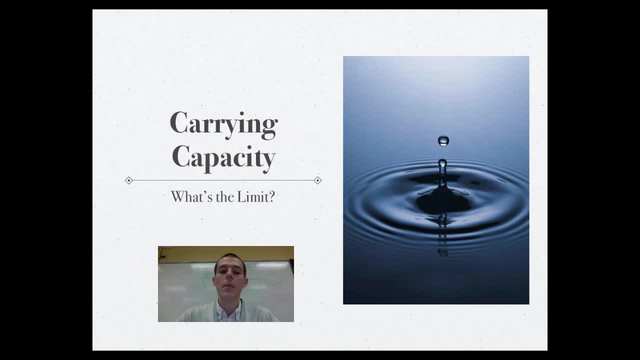 country, demographers can tell a lot about the quality of life based on the life of a baby and the life of the individual as a whole. and, kind of finishing up here, demographers talk about carrying capacity. all these things that I've talked about so far are looking towards carrying capacity, which 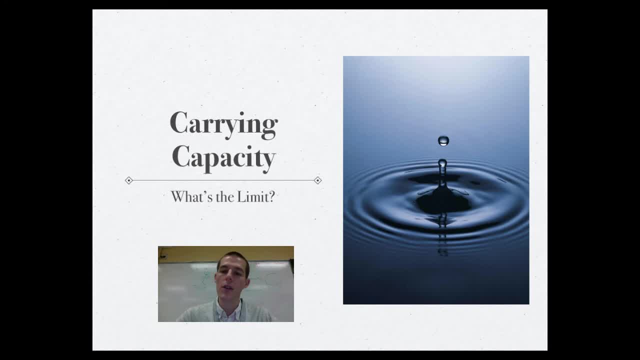 is basically the question of how many people the earth can support, and there's a lot of argument that goes around about what will actually limit the growth of the human population. will be water? will be space food, non-renewable resources, general conflict, the ability to get rid of waste? we don't really know, but we do. 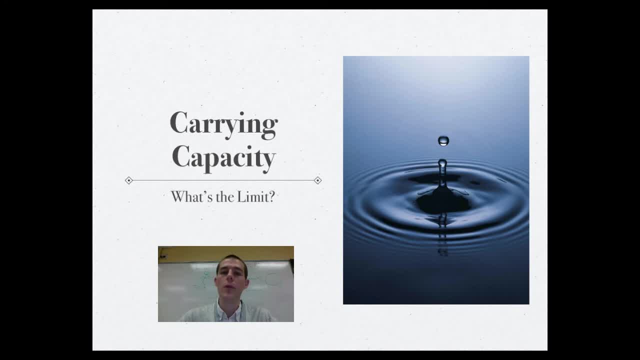 know from studying populations that every population on earth has some sort of carrying capacity and human population has been able to rock up forward and growth for so long with our ability to advance technologically that we're not quite sure where the carrying capacity for the human population is something that is. 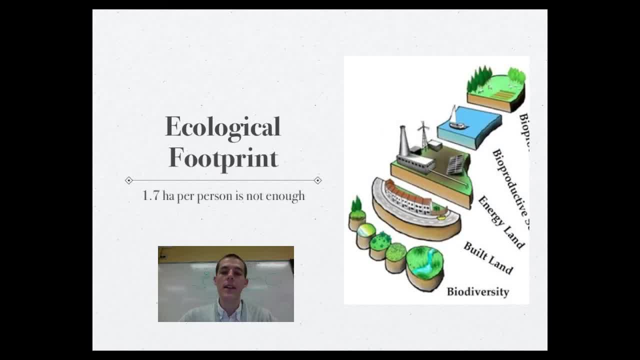 still an active debate, and one of the things that people use in this debate about carrying capacity is ecological footprint. ecological footprint basically talks about the land area and water area needed to support the lifestyle of a person, so that would be provided resources for the goods they consume. 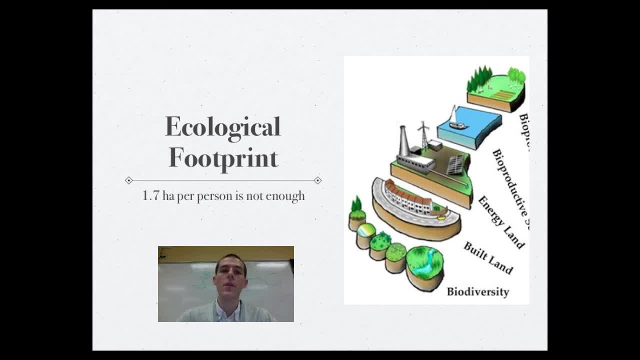 food energy also provide space to get rid of the waste. Now, if you take the land that is usable for all of these purposes, around the world divided by human population, it says that there should be roughly 1.7 hectares of land per person. 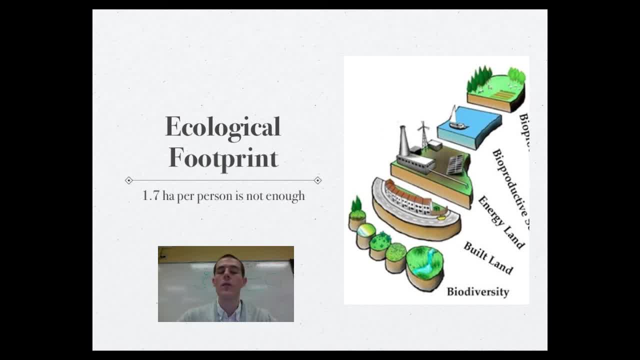 In some developed countries such as America, the average person uses roughly 10 hectares of resources. So you know, based on where you live, your- I guess- consumption and ecological footprint is going to be much bigger than if you live in somewhere that is less developed. And